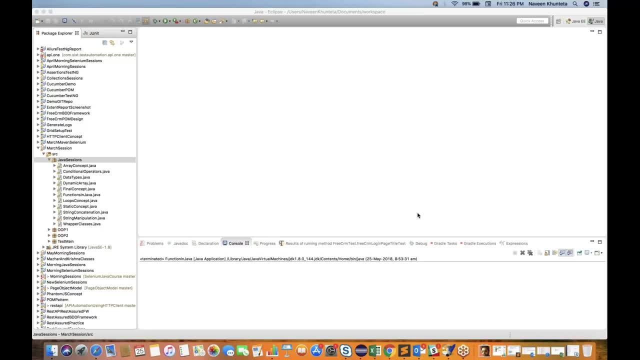 So what is the purpose of encapsulation and why do we use encapsulation, and what is the exact implementation of encapsulation? What are the advantages of encapsulation? We will cover those things. Encapsulation is one of the properties of, you know, one of the feature or one of the 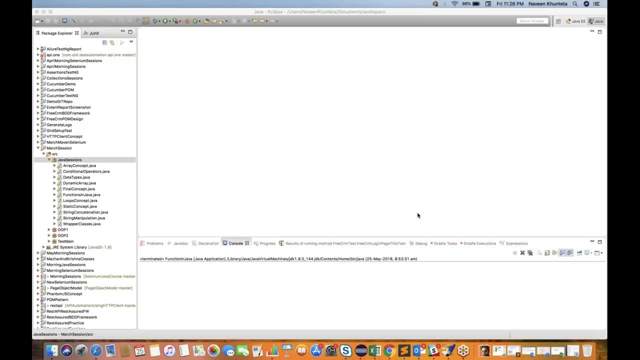 characteristics of object-oriented programming language. So in Java tutorial we have covered abstraction, we have covered interfaces, we have covered polymorphism, we have covered inheritance right. So one of the factors is that is called encapsulation. Okay, so what do you mean by? 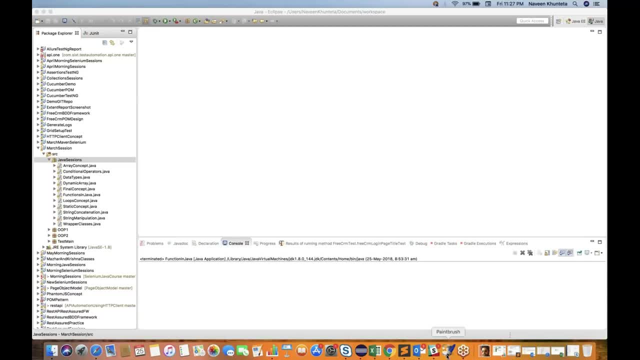 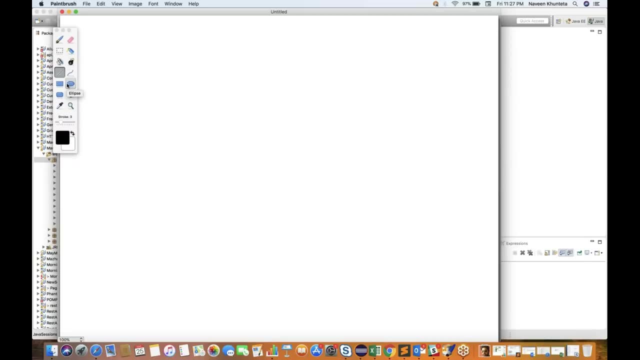 encapsulation So quickly. let's start with encapsulation. So what do you mean by encapsulation So quickly? I'll show one diagram for you guys. Let me open that. So encapsulation means you guys to hide your data members. Okay, to hide your data members. What do you mean by data members? 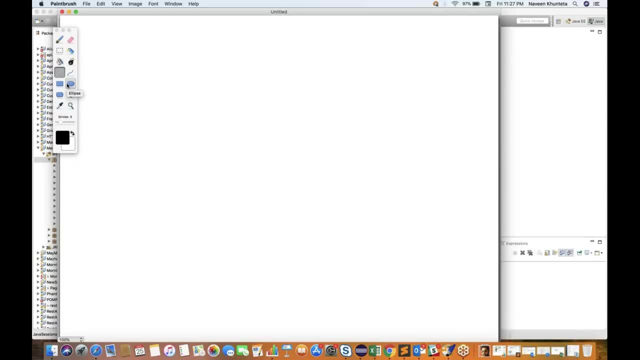 Data members. Data members means it can be a method, it can be a variable. So we define the variable as a static in nature. I mean private in nature, so that from outside of the class no one can access it. Okay, so that's why this is also called data hiding. We are just 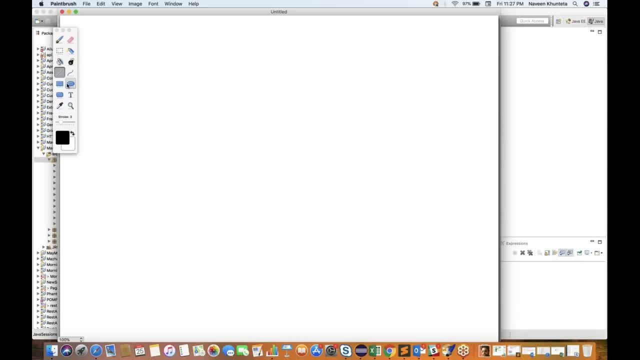 hiding the actual implementation. Okay, that, what kind of actual implementation is available in that particular class, So that from outside of the world no one can see that because we will declare as private variable Right? So encapsulation simply means the binding, your fields and the 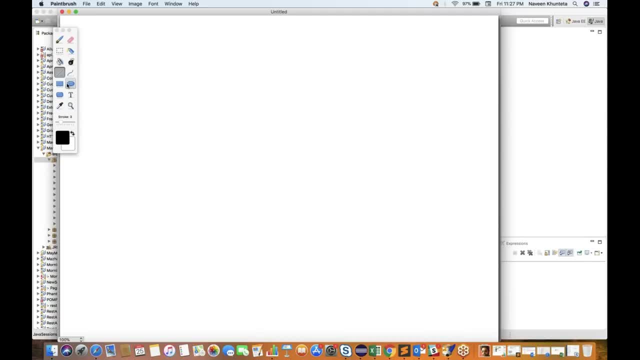 methods together. Encapsulate means combine the binding. Okay, that's why this is called data binding as well. Right? So let's see, I have this particular class. I have one class is available. Let's see my class name is you know? 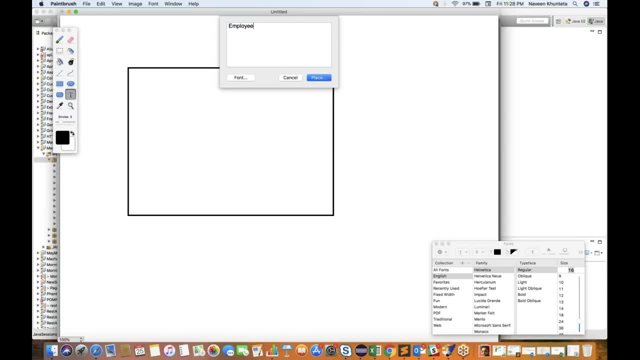 employee class, Employee class is there, So this particular class having some different standard methods or variables, one or two or three or four methods. four variables are there, let's see, and all are private variables And some methods are available. Okay, one, two and three, four. 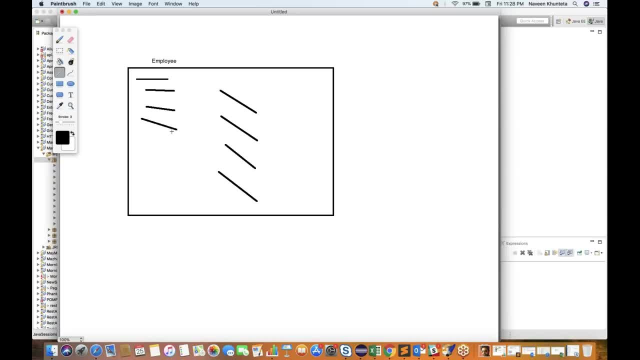 methods are available. So these variables are declared as private variables. Let's see some secure information I don't want to share to outside of the world, Right? So in that case I'll declare these variables as private variables and I'll declare some getter and setter method. Okay, 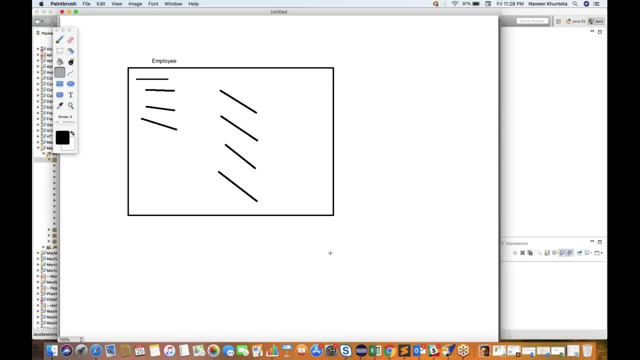 so that I can access and I can set the value from outside of the class as well. So let's see, one guy is sitting over here as a user- Okay, number of users are available over here. this user, Okay, Trying to access these variables directly. they cannot access it, they just need to call these. 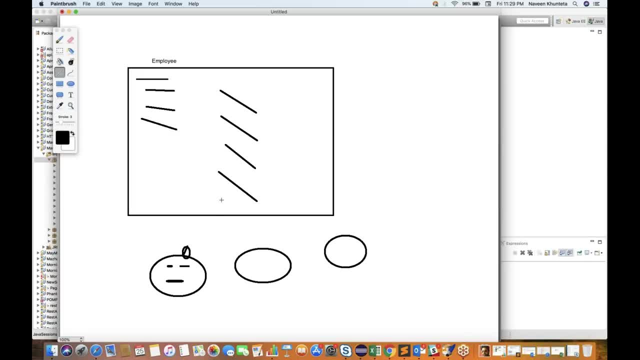 okay, call these methods Okay, from here to here, and these methods will call these variables Okay, So that we will get through these methods. we will get the information about, okay, all these variables, but we don't know what exactly the actual implementation they have done. 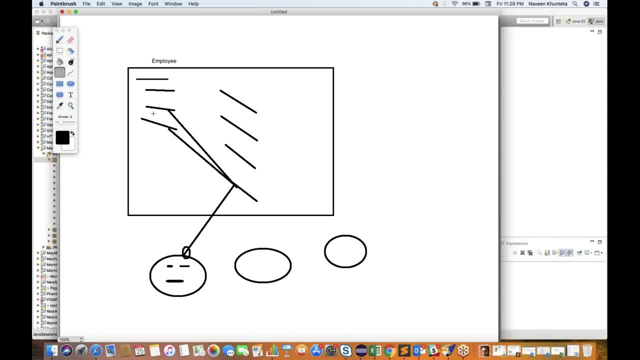 internally Right. So that's why, for security point of view, for hacking, a prevention point of view, we use encapsulation. Encapsulation is also called data hiding. it means no outside class, no one from the outside class can access the private data members. Private data members: I'm. 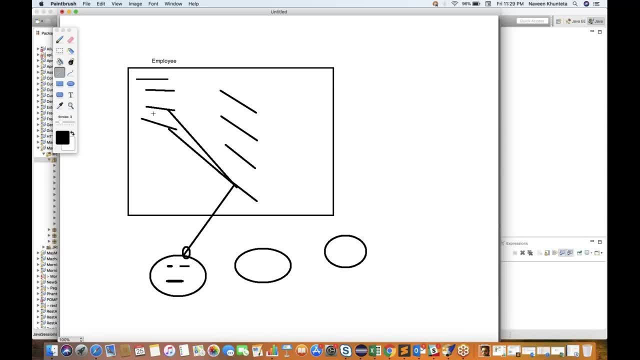 talking about here is private data variables of the class Okay, no one can access it. Let's try and give you an example: that social security number or very confidential information, or maybe your account number, I will declare as a private variable in this particular class, Right? So if 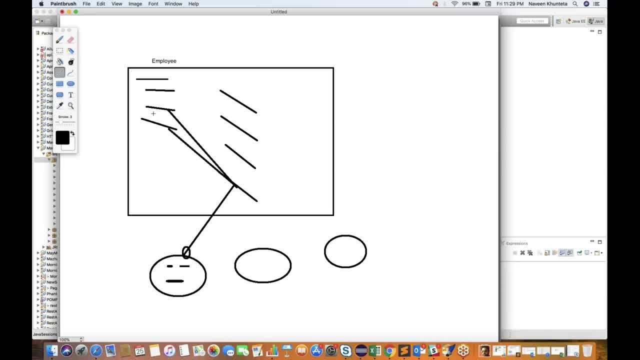 you really want to access it or you want to just get it, just get through these methods, But what exactly? the actual implementation, the actual logic I have inside the class, inside the methods, okay, the outside, this particular user, external user, they won't be able to see, they won't be able to access and they. 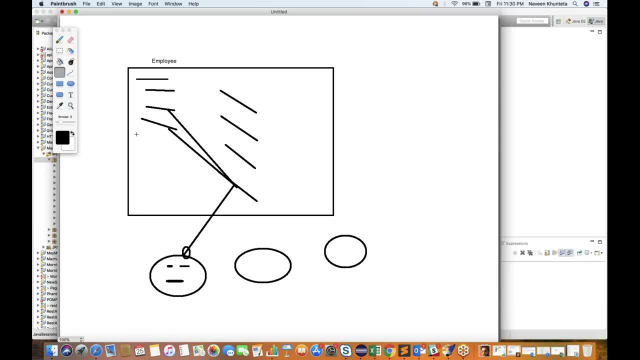 won't be able to change it also okay, like that. so so this is called encapsulation and we will talk about private property also. that okay, in this particular concept, in encapsulation that, what do you mean? that private as well, right, so let's create the same thing in terms of Java. so what I'll do, I'll. 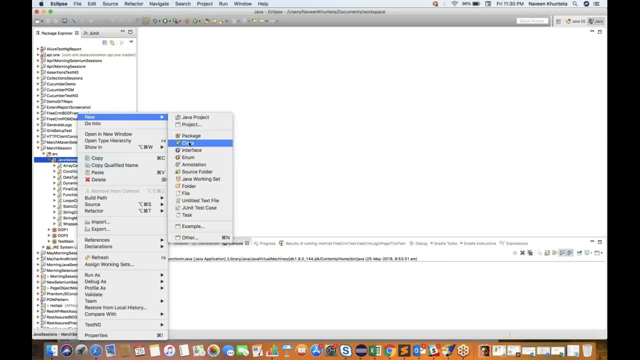 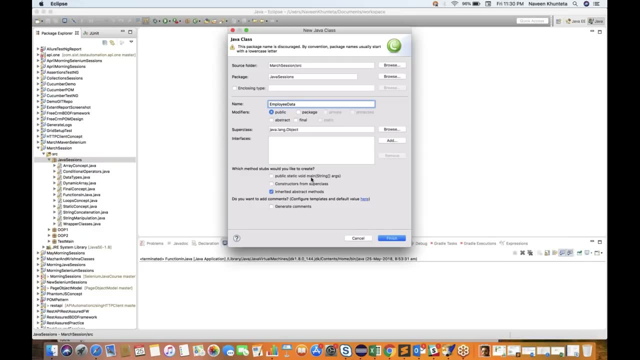 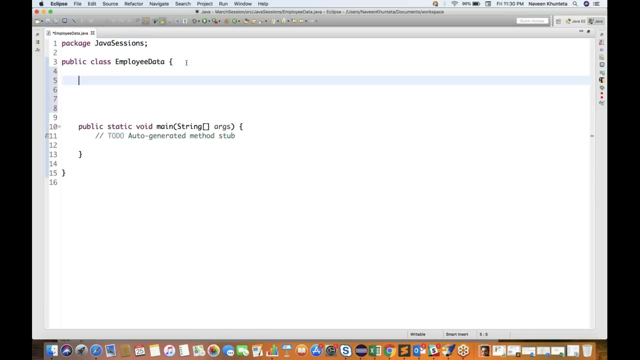 simply create a class. let's see. my class name is employee data and select the main method, click on finish and what I'm gonna do inside this particular employee data class, I'll declare three instance variable or three class variable, let's see. and all these variables are private variables, so private. let's see. 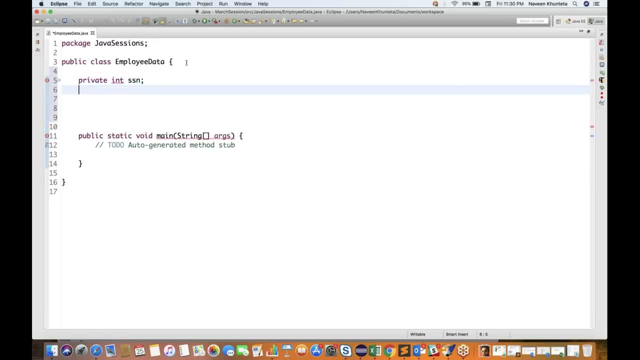 int sl number, okay, and then I'll declare variable that is string, employee name, right? SSN number means so social security number or something like that. and I declare one more variable. let's see private int- employee age, right? so these are the three private variables, two integer and one string. 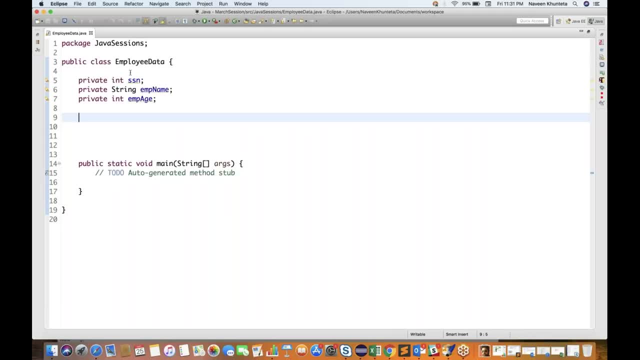 variable I have created. now I have to define. these are called private data variables. okay, fine, now I have to define some getter and setter. get a ren閉喔 method I have to define. so how to create getter and setter directly. so you just need to right-click over here and simple go to. 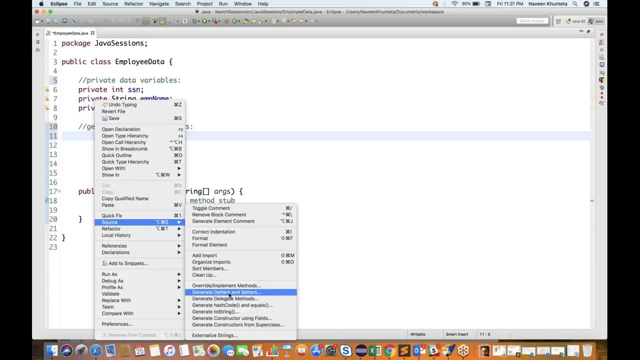 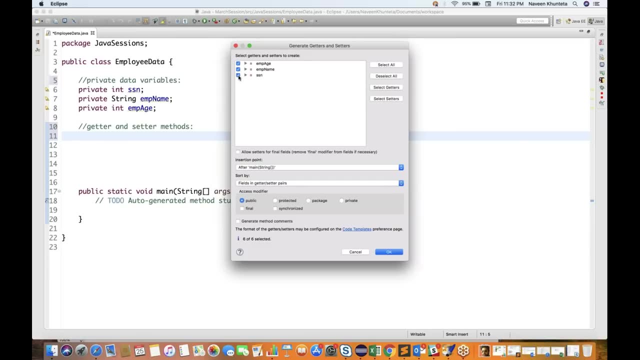 go to source and you can see that there are about six26 Write効 to address a and you can see that getter and setters. right, so click on generate getter and setter. for all the variables i want to create: getter, getter and setter, and these getter and setter will be: 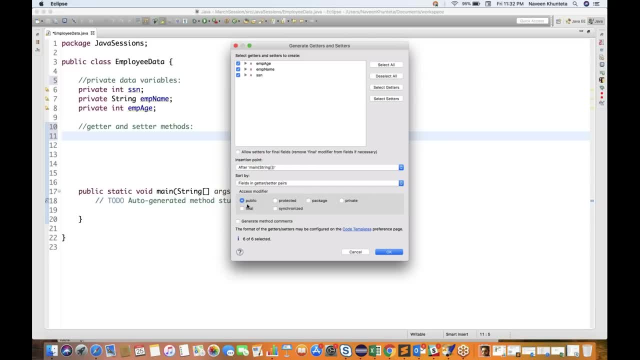 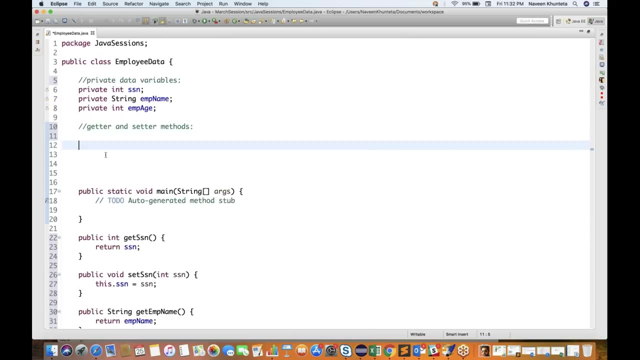 public in nature, because if you declare them private then no one can access these methods. okay, within the class only i can access. but i wanted, okay, these getter and setter for all these private variables can- x, can be accessed from out of the world as well. so click on ok, so you will see that number of. i'll declare like this: 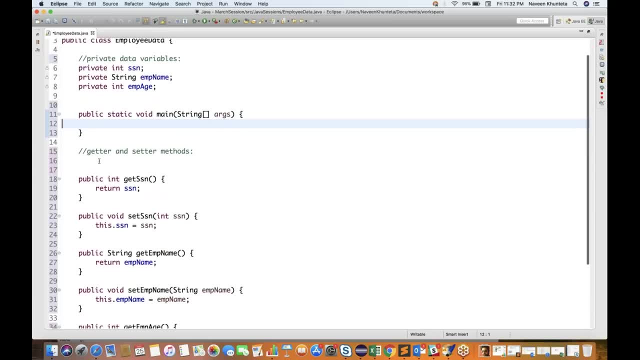 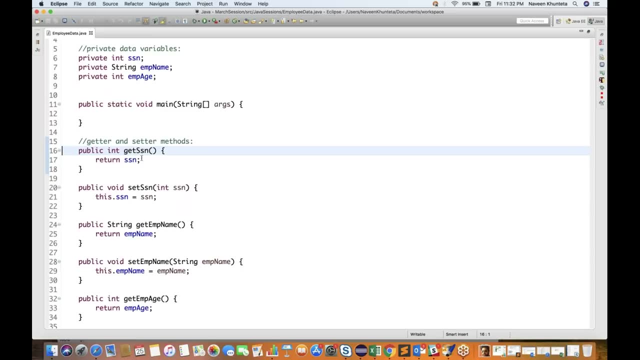 okay, so getter and setter methods got created automatically, so no need to write the code. getter and setter- simple, you can generate directly from the source. so if you see, for ssn we have this get method and we have set method. so inside the set method we can. 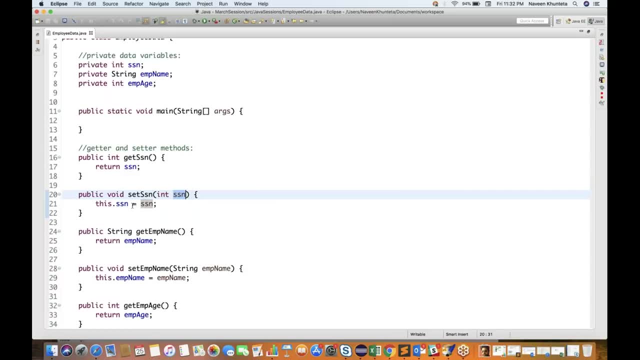 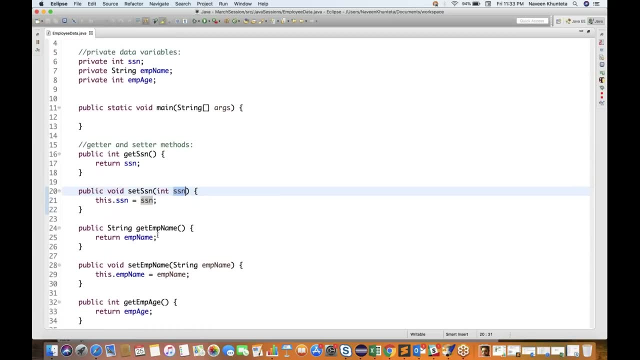 okay, uh, set this particular method, we will pass one ssn number and this dot ssn means this dot particular global variable is equal to whatever the local variable that we are passing over here. same thing for get employee name. so we have: first we will set and then we will get. 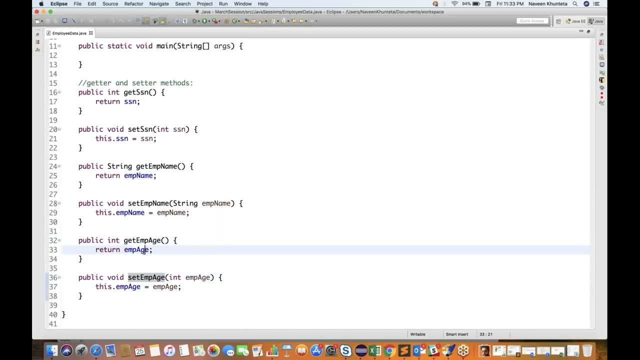 same thing for get employee age: first we will set and then we will get the same age that we are declaring. we are sending to this particular method right now what i'm gonna do. so always remember the example of encapsulation in java: how to implement encapsulation in java. so, to implement encapsulation in java, the first thing is that you 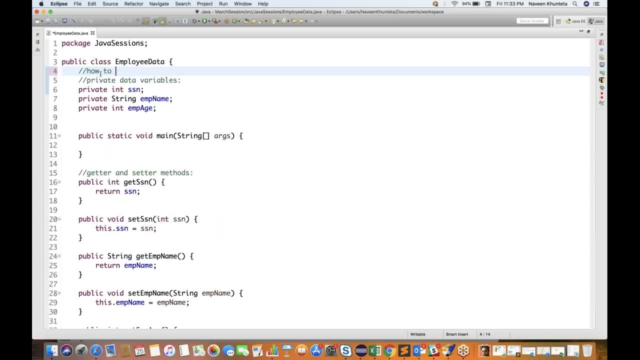 have to. so the concept here is that how to implement, okay, encapsulation, how to implement encapsulation, encapsulate, me. encapsulation mean encapsulate in a particular capsule, in a particular class entity- okay, and capsulation, okay. so what we have to do? first, make the instance variable, private, so that 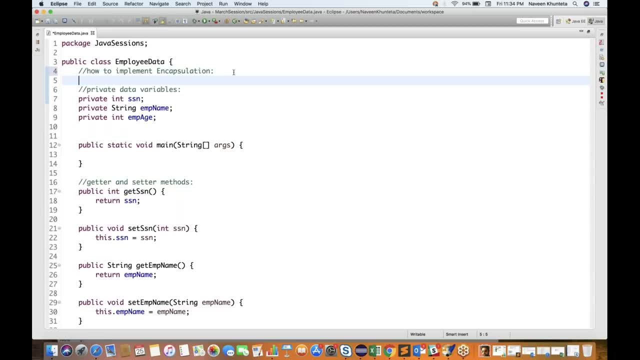 they cannot be accessed directly from outside of the class. okay, so private data variables we have to create so that, okay, these, I'm writing the notes for you guys- so that these variables cannot be accessed directly from outside the class. okay, directly from outside the class. so this is the first step that we have to. 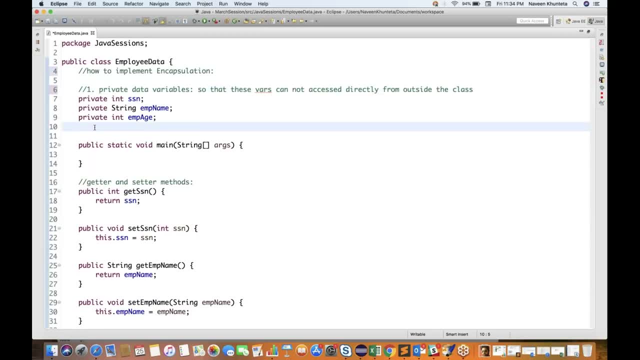 create right. second thing, what we have to do, that you have to create getter and setter. so this is the second step: that we have to create that getter and setter method right in the class to set and get the values of the fields, to set and get the values. 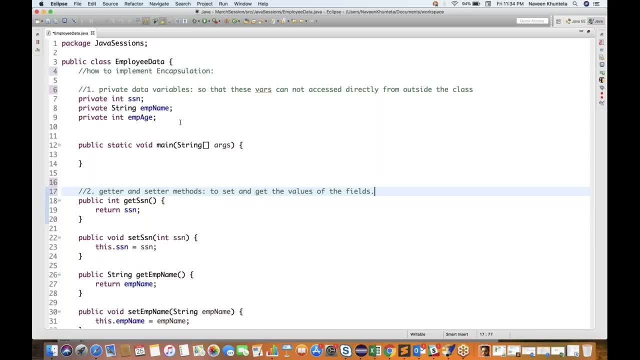 of the fields. fields means these particular fields. three variables are there, right? so this is how we implement encapsulation. now let's test this particular encapsulation. that what I'm going to do in this particular main method. I'll do one thing that I'll create the object of 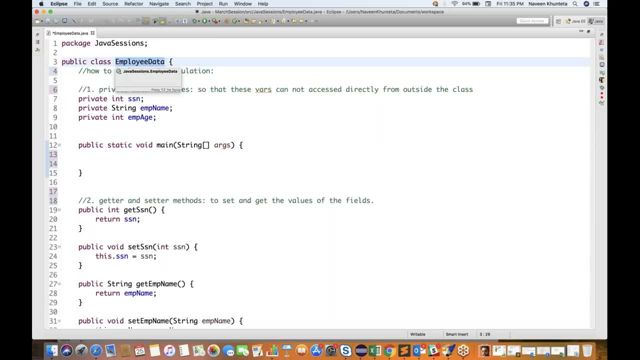 because I have to access these methods, so I have to create the object for this particular class, because these are non-static, so have to create the object. simple OBJ. or let see: EMP is equal to new. okay, class name. and then what I'm going to do: I'll set all these variables- okay, the variables value- by using this. 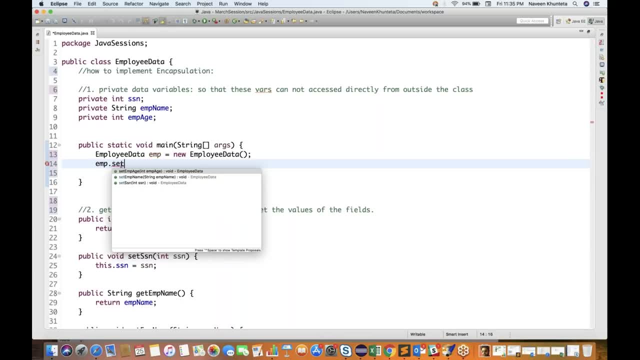 emp dot. set SSN, or. let see. first I'll get the employee name. I said the employee employee name is: let's see. my employee name is: uh, let's see. instead of Naveen, let's write some proper name: Tom, okay, Tom Peter. I'll write BMP dot. I'll set the age: okay, set employee age. 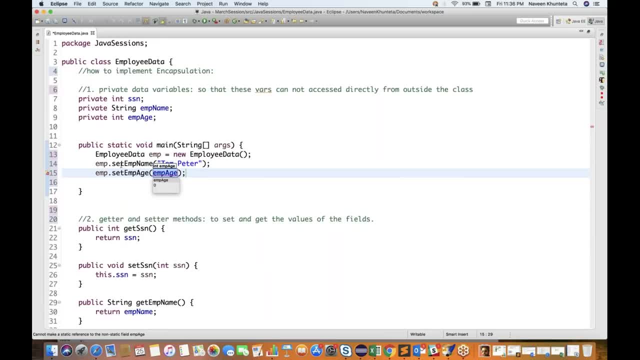 and employee age in. let's see, employee age is 25. okay, that is an interior variable. and employer dot. we have SSN number, so set SSN, so we have to provide the SSN number and SSN number. let's see some six digit number. I'm writing that: okay, uh, one, two, three, four, five, six, some six digit. 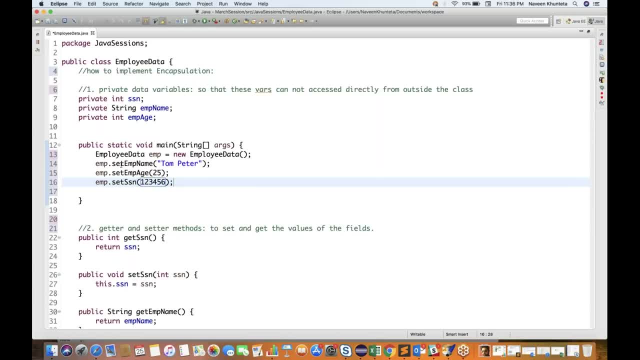 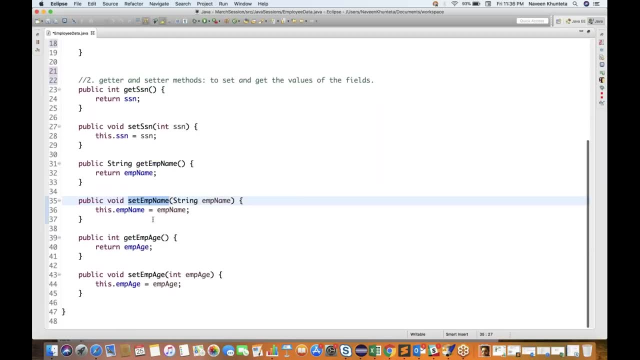 number. let's see something I'm passing over here. right, so I have set the value, okay. so what exactly it will happen? employer dot set employee name, so employee name, it will jump to employee name. it is by default. oh, one, two, three, four, five, six. one, two, three, four. so we are going to write. 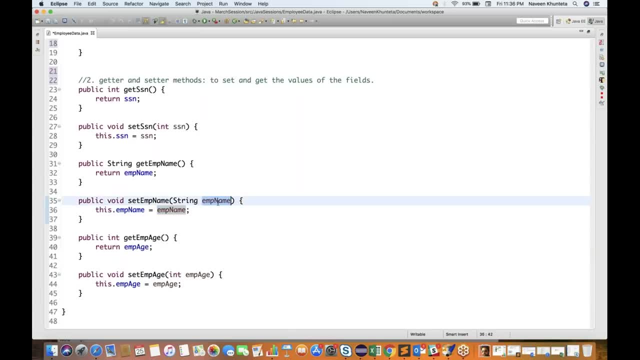 Isn't this? S is equal to one, one, two, three, four, five s. let's, we will give a value set employee name. it is equal to one, one, two, three, four, five, six. that's it for this class, every one of the two dot classes. right now I will name my these array name. I have set my third. 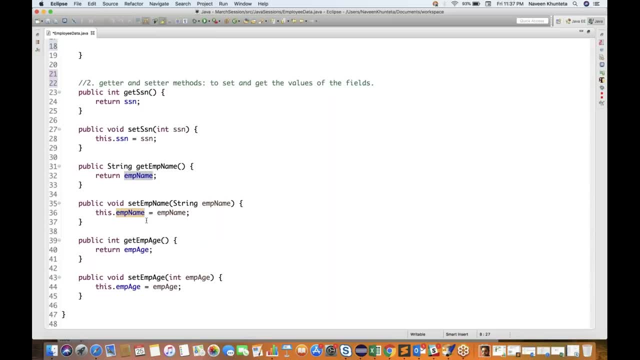 word into my name, so you can just importance. oh sorry, sorry, I have this that I have done. let me underline that the class is inside, but this class, inside the class you will create, class variable is equal to local variable and local variable the value we have passed. tom peter. 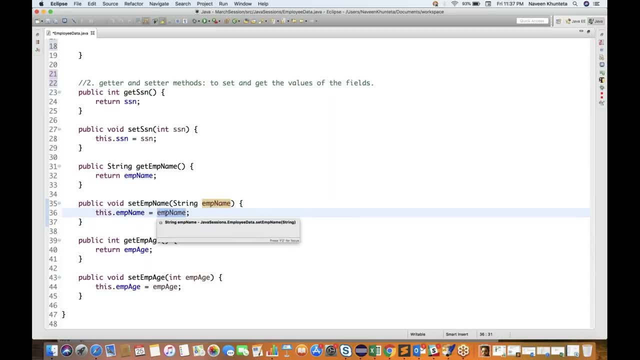 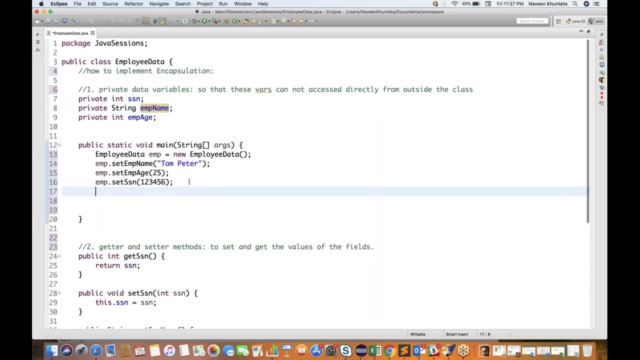 will be given to this guy, will be given to this guy and this guy, tom peter, will be given to this class variable. so this dot class variable is equal to local variable. so employee name: the class variable will be set to tom peter now. so the value of employee name will be tom peter now i just need 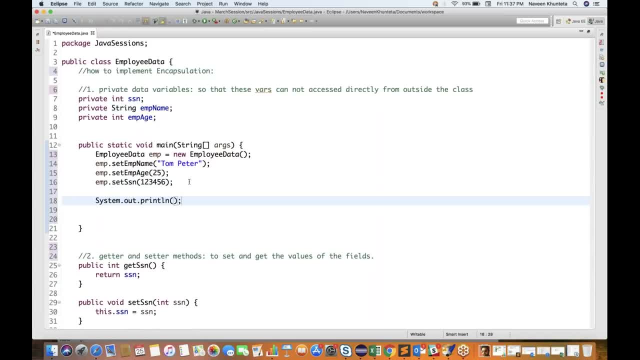 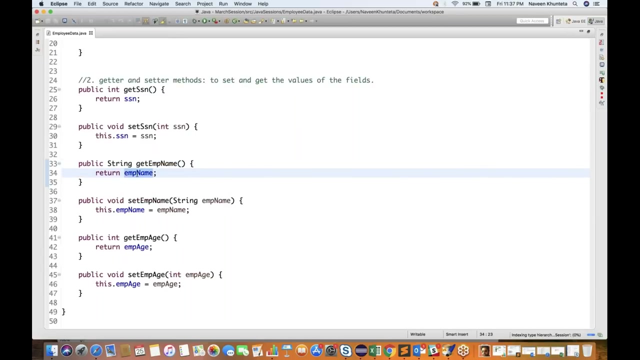 to get the value. so i'll just print on the console: system: dot out, dot pinterest. let's see. i'll write like this: employee name is uh, emp dot get name. right, so we will call this method: emp dot get employee name. so get employee name will return this employee name. and employee name is what the class variable that we have. 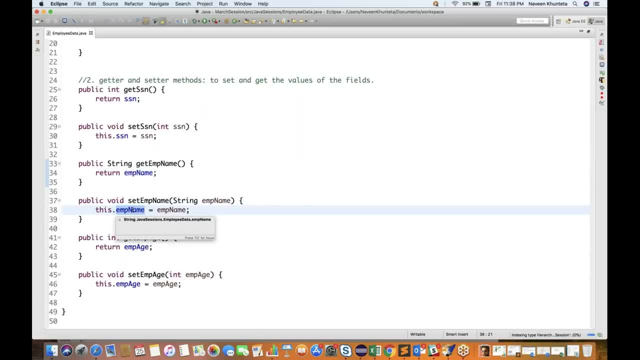 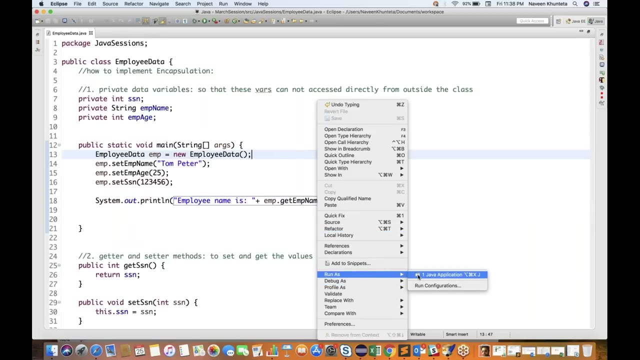 already. okay, set it to tom peter, because we are passing tom peter to this guy, tom peter from this guy to class variable and we are returning the class variable only so we will get tom peter over here. so let's see, let's run this program and let's see it is working or not. so run as java application and you will see. 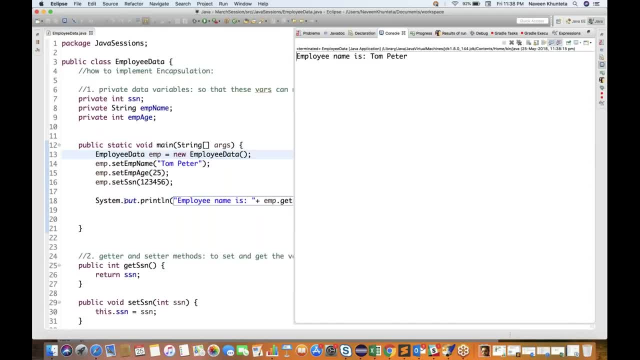 the employee name is tom peter. same thing. we will get the age and ssn number as well. system dot out of println. let's see i'm printing the ssn number. or let's see the age. employee age is emp dot get employee age. so let's see: are we getting the employee age or not? so yes, employee. 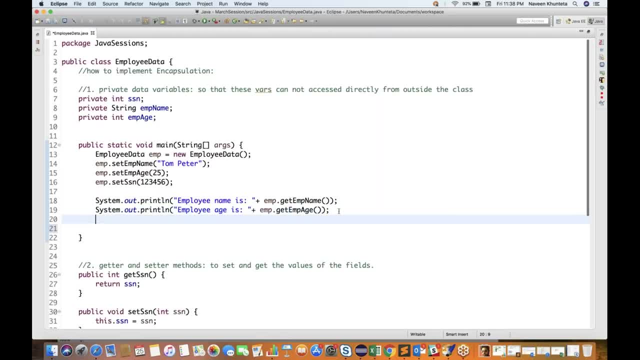 age is 25, same thing, for we are printing it for ssn number: employee. ssn is employee dot. get ssn. so let's see we are getting the or not. yes, we are getting SSN one, two, three, four, five, six as well. right, so this is how we achieve, okay, the encapsulation. so encapsulation in this. 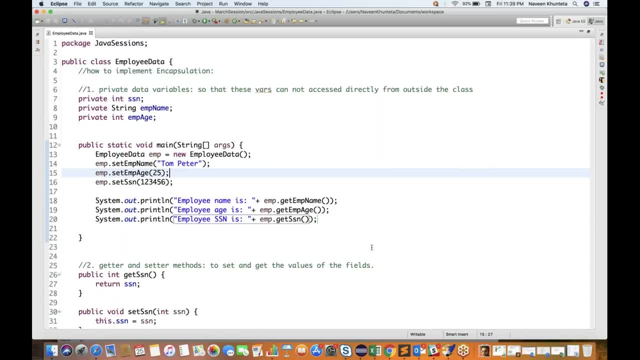 particular example that we have seen. the three data members are there, or we call three data fields: are there SSN number, employee name and employee age right and we are using the access modifier as private so that outside of the class no one can access. okay, from outside the class no one can access these private. 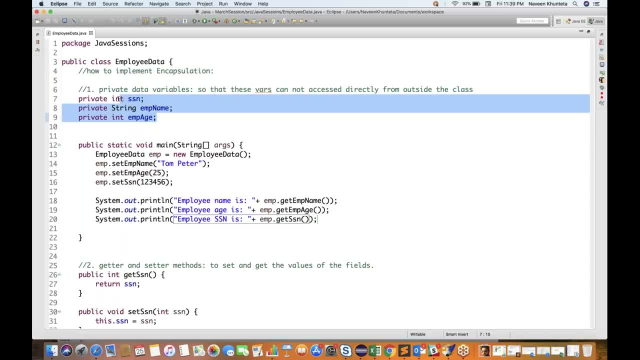 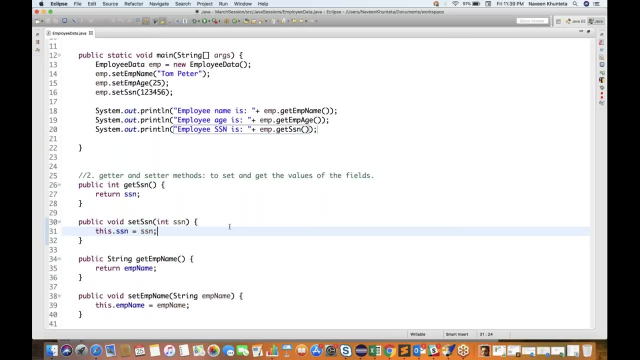 variables. if you really want to access these private variables, we need to define the getter and setter, right. we need to define the getter and setter over here, so you just set the value and get the value. set the value and get the value. this is a property of getter and setter right. so in this example we have 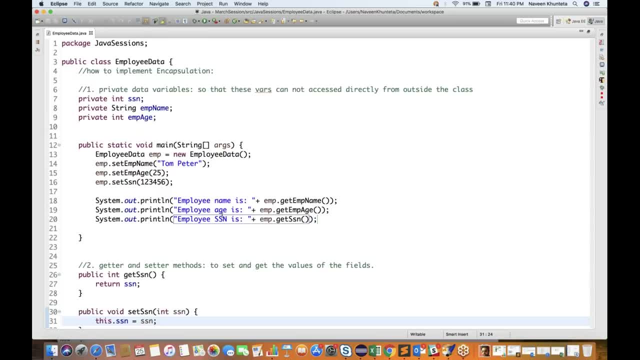 seen three private variables which cannot be accessed directly. these variables can be accessed via public methods. so always remember getter and setter will be public always. if you create your getter and setter private, then within the class only you have to access. then what is the purpose? from outside of the class you have to call these methods instead of these variables. 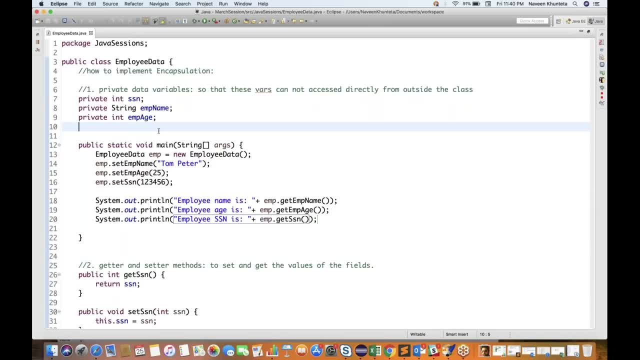 so always remember, in encapsulation, variables should be declared as private and the getter and setter should be declared as private, so that by using this private methods, we will call these private methods so that we can access these. okay, we will call these public method so that we can. 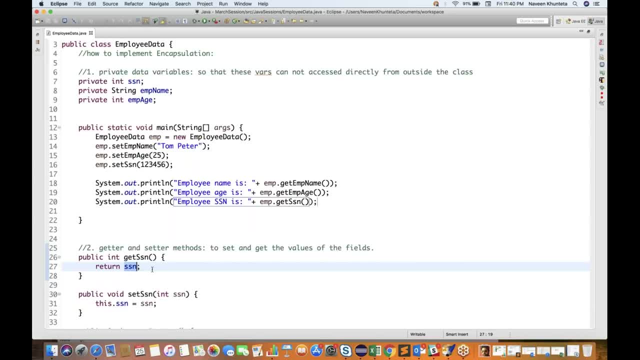 access these private variables. I'll repeat: in encapsulation we declared private variables and the public getter and setter so that from outside the class we will call these public get method and we will call this public set method to set the value and we will again call this get method to get the value as a. 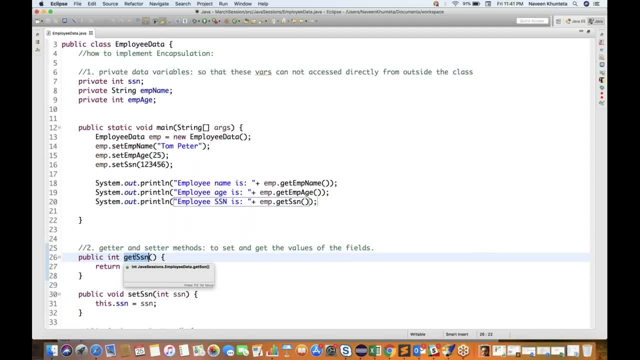 public, because this is public in nature, and then we can access from outside of the class also and we can access all the private variables. so this is the property of encapsulation right now. what are the advantages of okay encapsulation? it improves the maintenance of the code, the 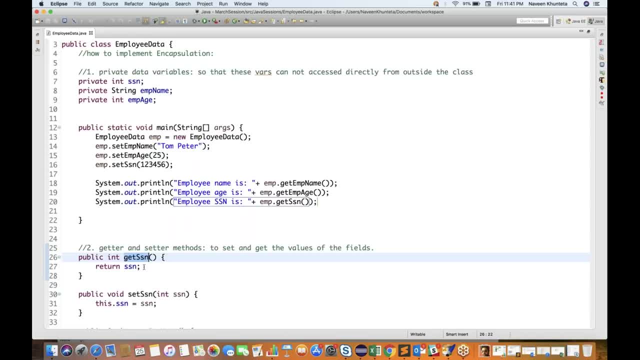 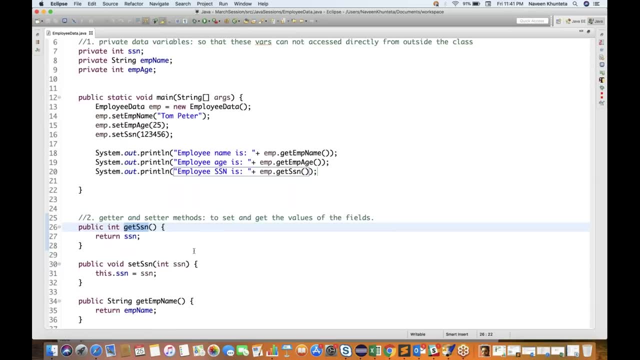 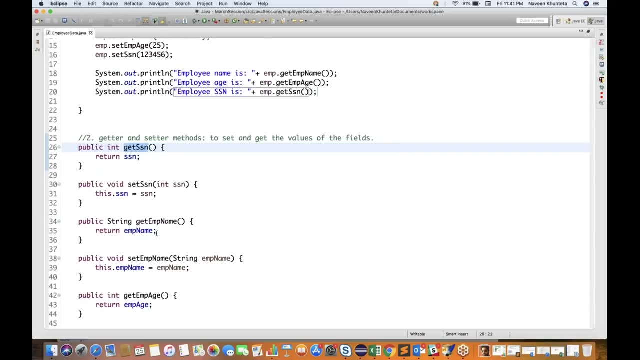 flexibility and the reusability right. let's see in this particular example the implementation code of set employee name or set SSN security name. okay, can be changed at any point of time. we can change the logic internally, but from outside the world, the external user, will never see what exactly the 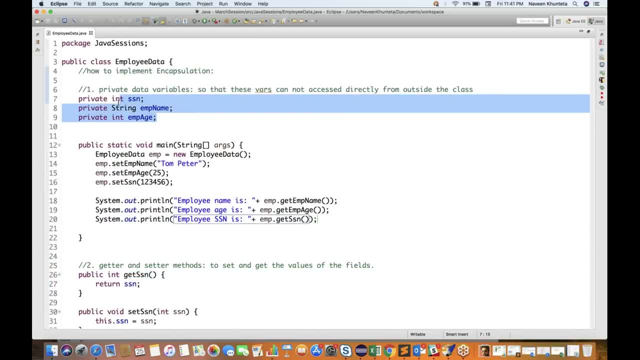 implementation. how many variables and what are other variables are available. the private variables are available. okay, so this is this. information is hidden, right, and you can change the implementation of all these getter and setter anytime, so it will give you a very good amount of flexibility and the 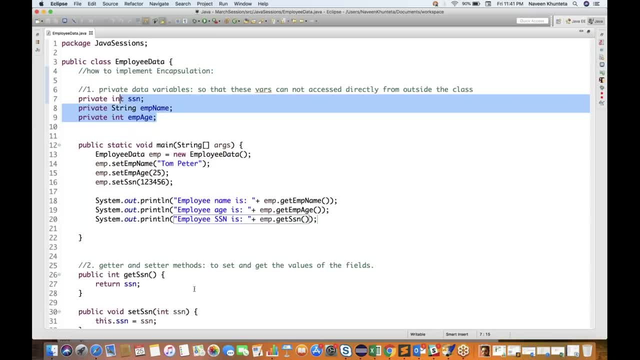 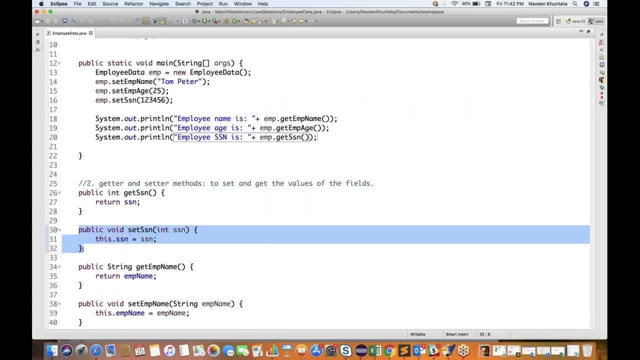 maintenance of the code, as well as the reusability as well, right. another advantage is that these variables can be always read only. okay, because you can be made read only if you don't define setter method. I want, I don't want to use set method. I don't want to use the. I don't want to set any method from. 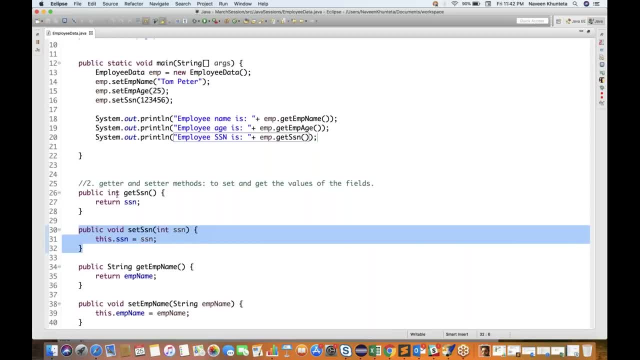 outside the world. so we can. we can have only get method, private get method, so that you can access these variables. that's it from outside the class. but okay, if you don't define the getter, getter method or setter method, if you really don't want to do that, just don't declare set method. we just declare the get. 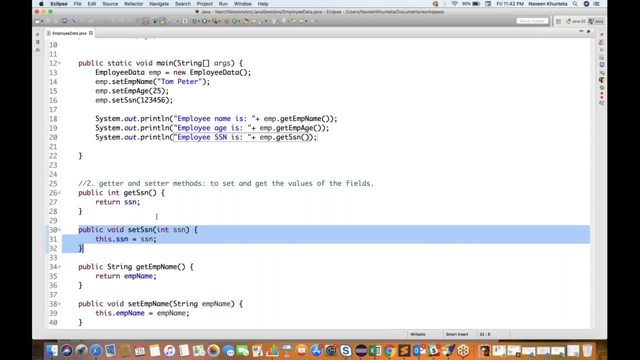 method so that we can access it right. apart from that, external user will never be knowing that what is going on behind the scene, right? how many private variables are there and how exactly the declaration and everything. they would only be annoying that to update a field- okay- using the set method and to read that particular variable using the get. 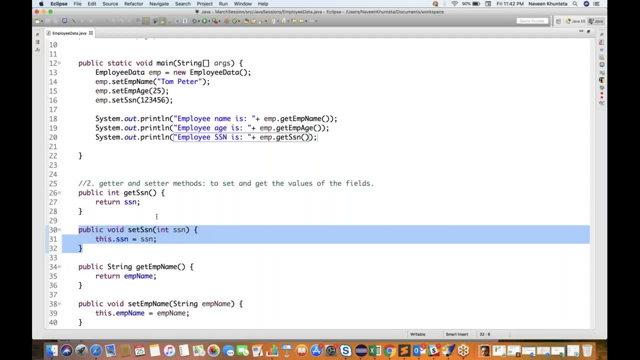 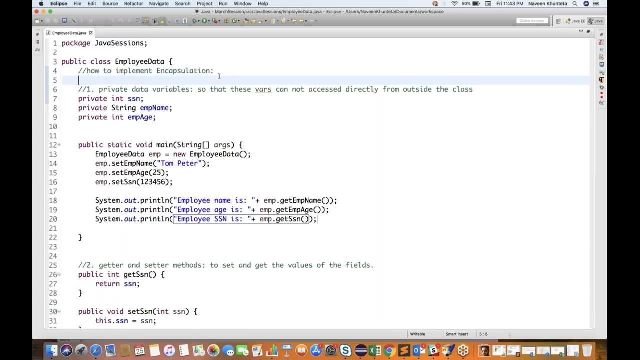 method. okay, it's totally hidden from them. so what exactly the implementation is, how many variables are there, is totally hidden to them. that's why encapsulation is also called data hiding. okay, guys, always remember encapsulation is also called data hiding, so don't be confused that people may. 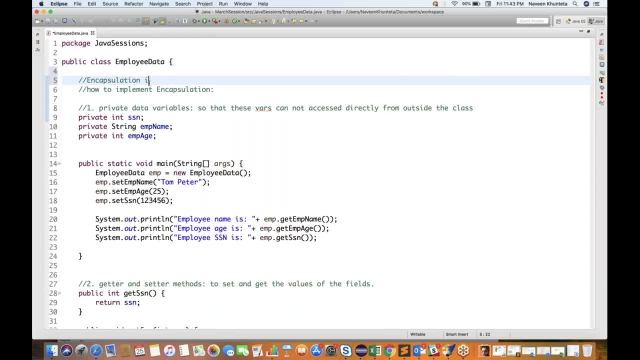 might ask at a time of interview: what do you mean by data hiding? so encapsulation is also called data hiding. okay, okay, one more thing, guys. okay, one more thing, guys. it's not compulsory to define getter and setter. always it's up to you if you. it's not compulsory to define getter and setter. always it's up to you if you. 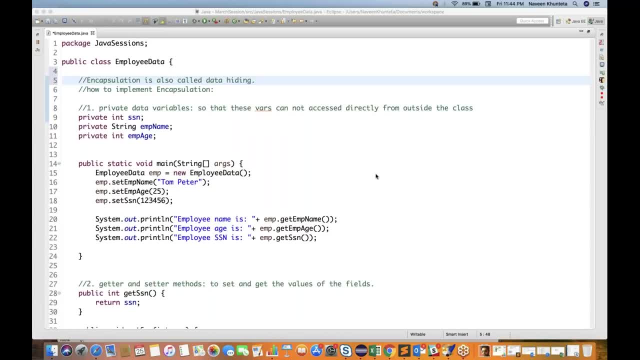 don't define any getter and setter, just declare private data variables so from from outside the class no one can access it right. so to provide the very high, high level security, now assume that SSN employee name and employee age or account number or employee salary- all these variables are publicly. 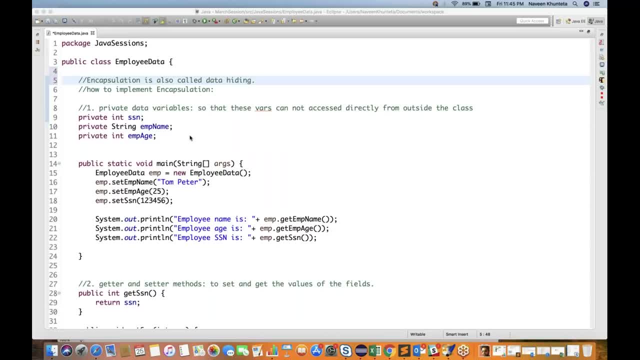 defined, anyone can access these information right. so, to provide the very some high-level security in Java, okay, we use encapsulation because you can hide and you can restrict access to critical data members. critical data variables: okay, in your class, which are defined, which improves the security okay. 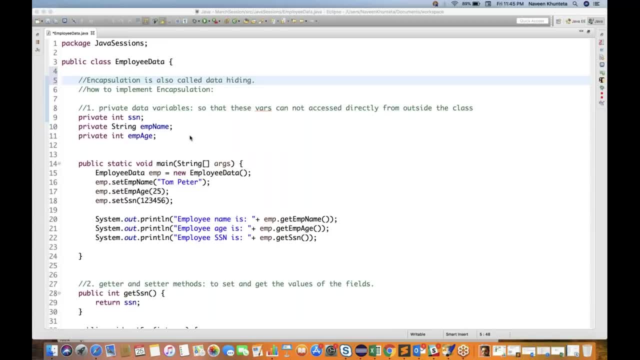 it's not compulsory to define this okay, getter and setter. but if you really want to access those private members, those private variables, in that case only you have defined public getter and setter method. so I would say public getter and setter method you have to define to access, okay, private variables, right? so